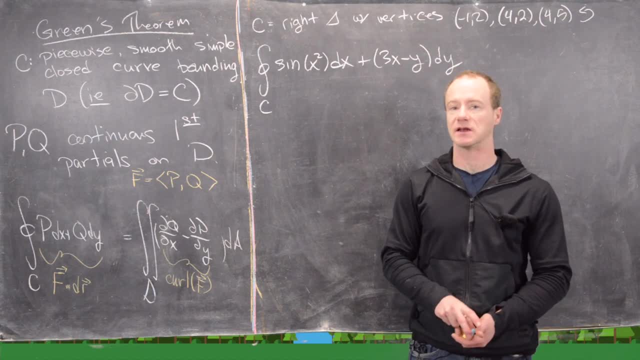 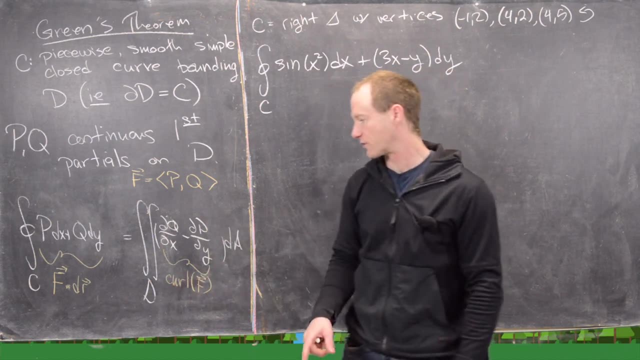 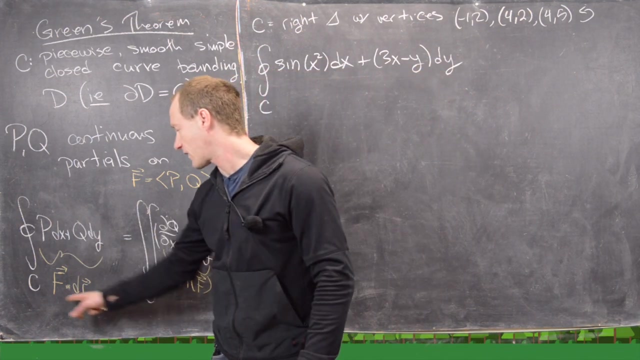 So F is a vector field with component functions P and Q. Then the line integral over C of PDX plus QDY is the same thing as the double integral over the region D of partial Q, partial X minus partial P, partial Y. And then also notice that this guy over here is just the line integral of F dot DR, where we've defined this F right here. 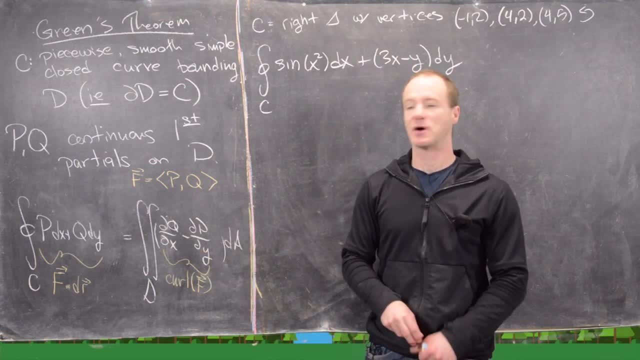 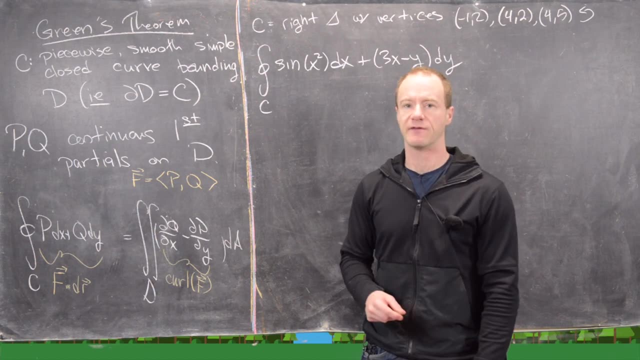 And then this partial Q, partial X, minus partial P, partial Y, is just the curl of F. It's this like curl of a two vector field. The curl of a three vector field is a slightly different definition. Okay, so the first example we want to look at is this one: 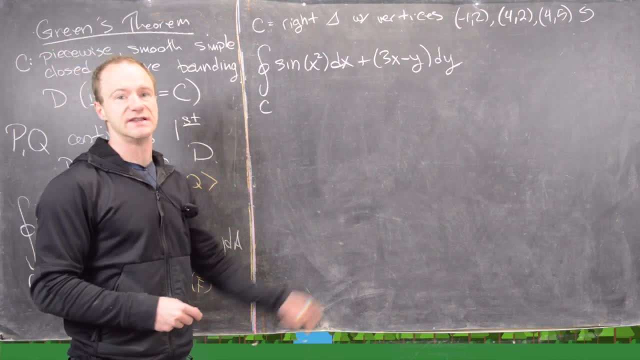 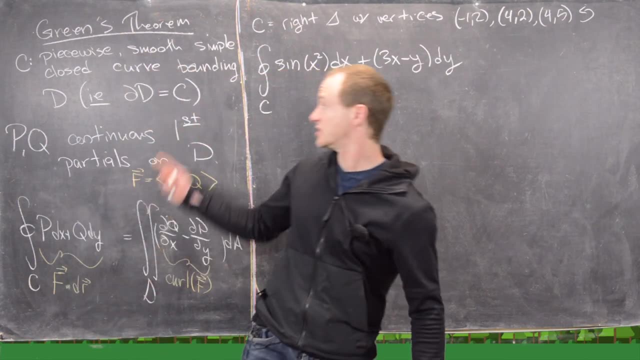 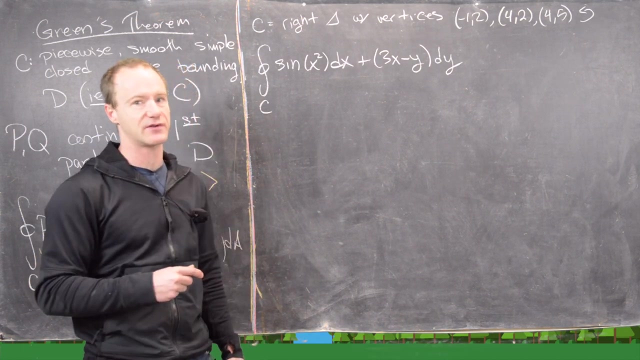 So let's see the right triangle with vertices. So we've got negative one, two, four, two and four five And we're orienting that counterclockwise. And I should say here this C has a positive. So that means if you're walking along C, the region that it's bounding is to the left. 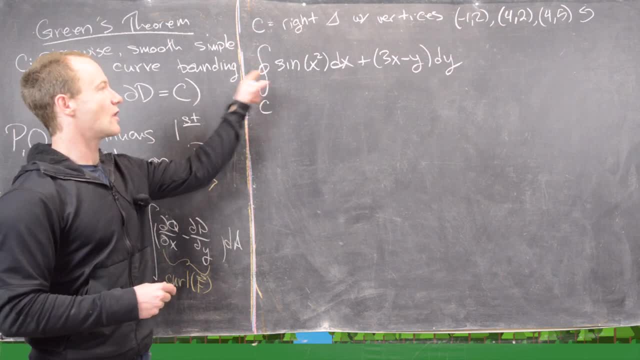 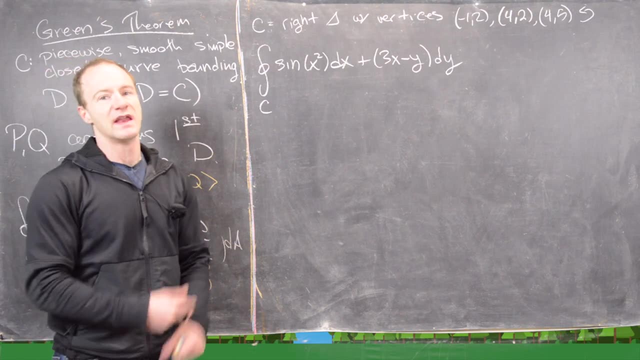 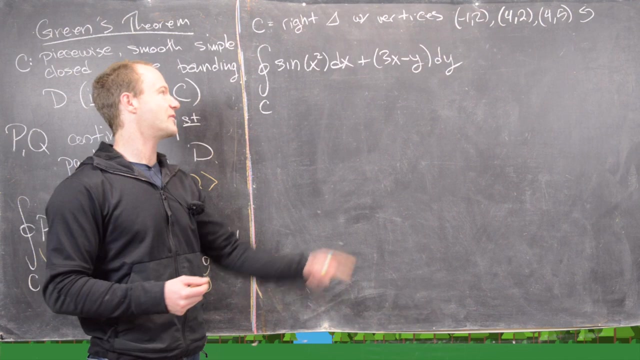 Then we want to calculate this line integral, So the line integral over this triangle of sine X squared, DX plus three X minus Y DY. Now we could set this up as a line integral and we would see that it's quite difficult to calculate. In fact I think you get a non-elementary function to take an antiderivative of, given that you have a sine X squared here. 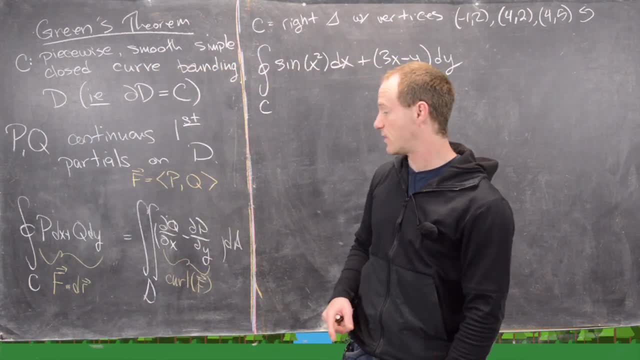 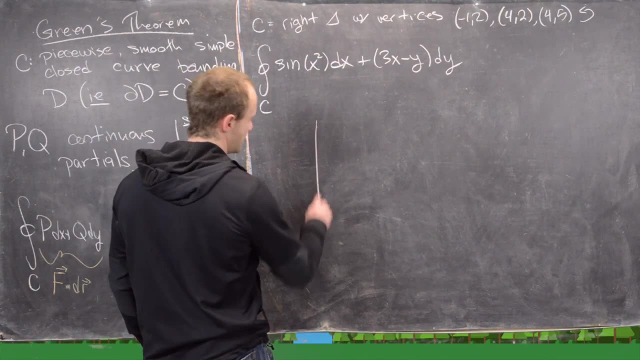 So we'll actually just use the result of Green's Theorem to put this into a double integral. So let's get an idea of what this picture looks like. So there's my X- Y plane. So I need the point negative one, two on there. 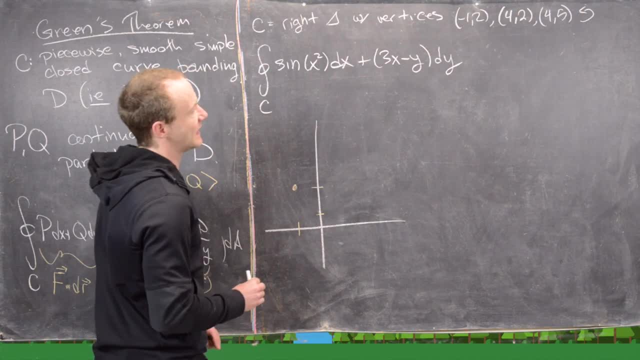 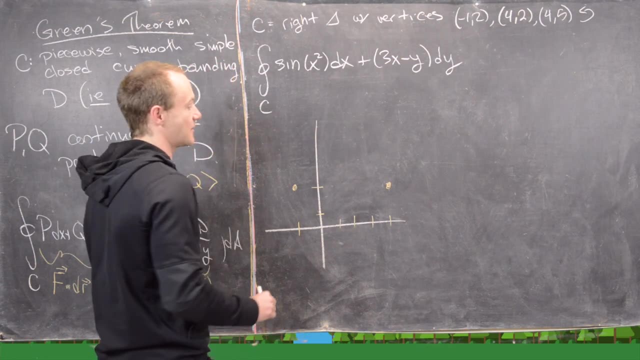 So that's going to be like right about here. And then I need my point four, two. So let's see one, two, three, four, two. So that's going to be right about there, And then four, five. 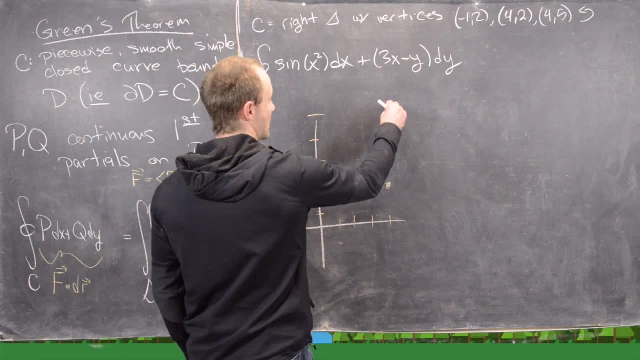 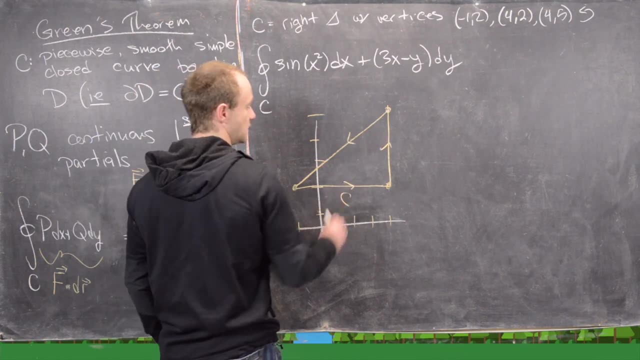 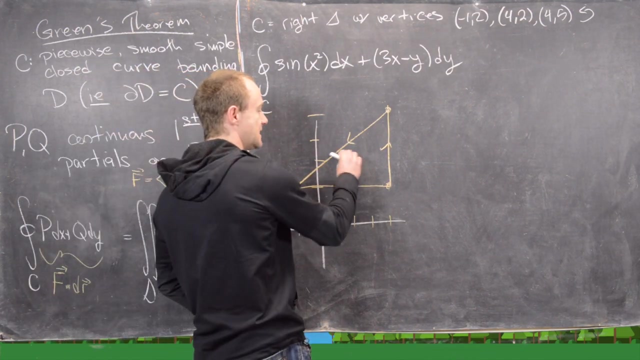 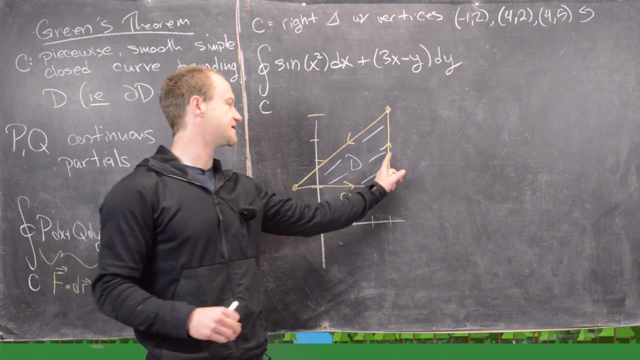 So three, four, five. So that's going to be right about up here. So there is my curve C, which is oriented positively, which makes the region on the inside D this thing right here, Okay. So what's nice about this is this is a horizontal line and this is a vertical line. 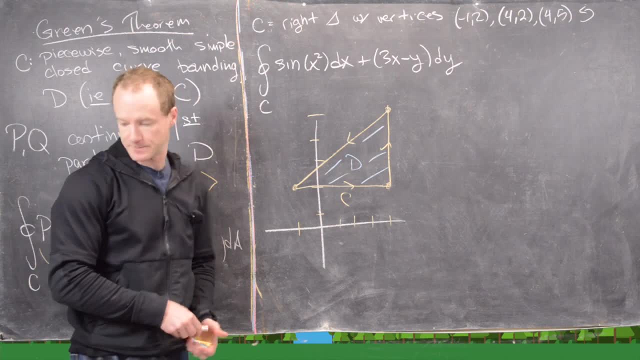 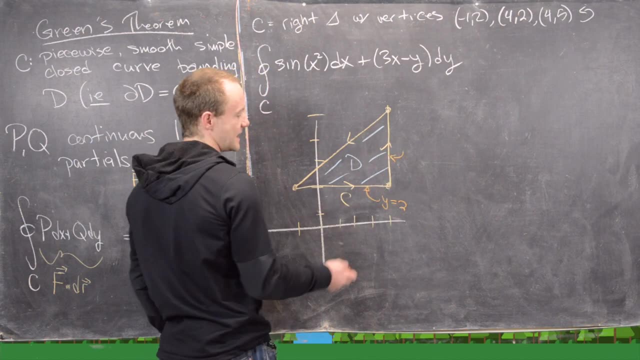 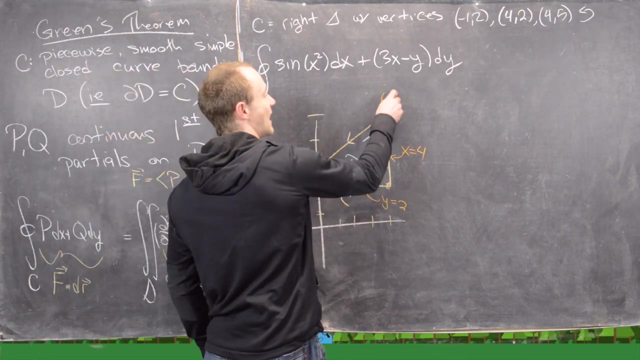 So that's going to make this setup of this double integral pretty simple. So notice this guy Down here is: the horizontal line y equals two. This guy right here is: the vertical line X equals four, And then we can use the fact that this is the point four, five. 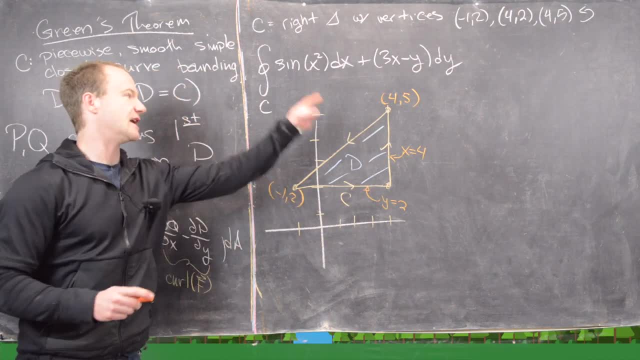 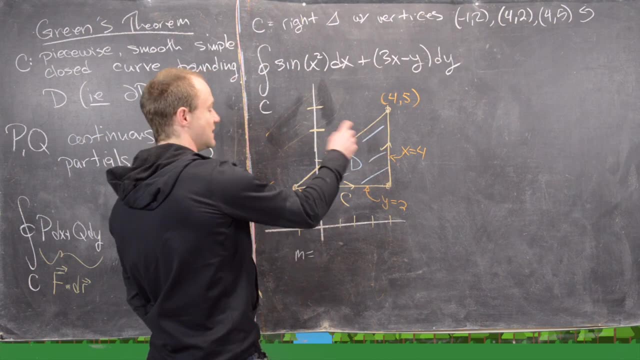 And this is the point, negative one. two, to easily find like a point slope form of this line. So notice, we need the slope first. So that slope is going to be the change in Y divided by the change in X. So notice, our change in Y is zero. 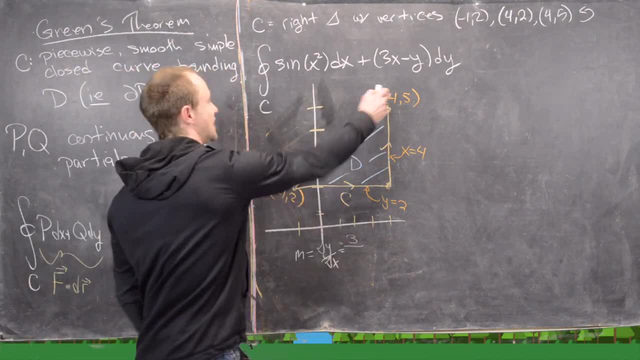 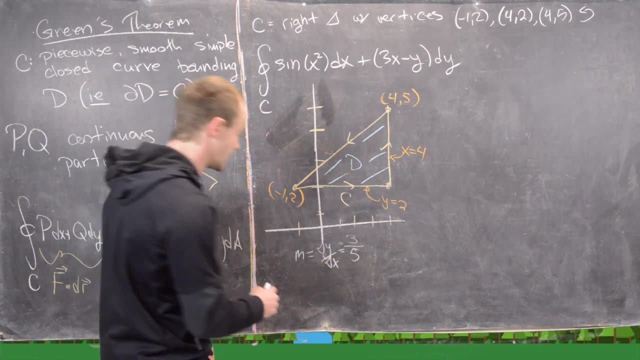 5 minus 2, so that's going to give us 3.. Our change in x is 4 minus minus 1, so that's going to give us 5.. So that makes our slope 3 fifths. The next thing that we can notice is that, using the point, 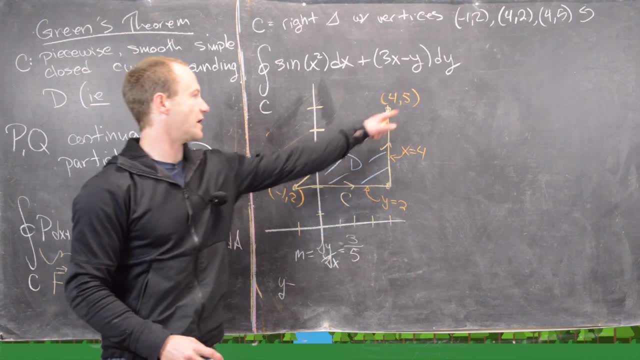 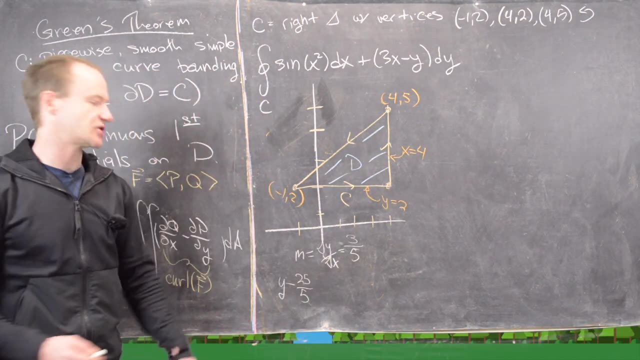 slope form. we have y minus the y part of the point. Notice, the y part of the point is 5, but I'm going to write that as 25 over 5 because I'm going to need like a fraction. So that's going to. 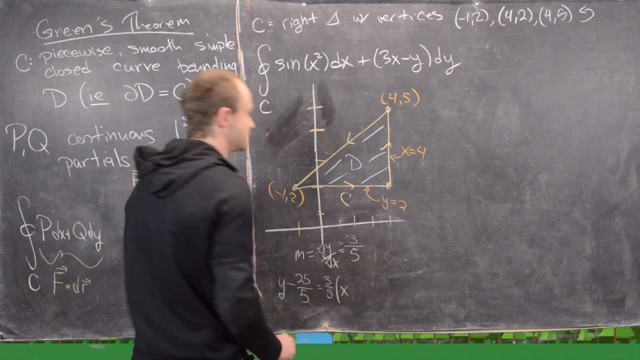 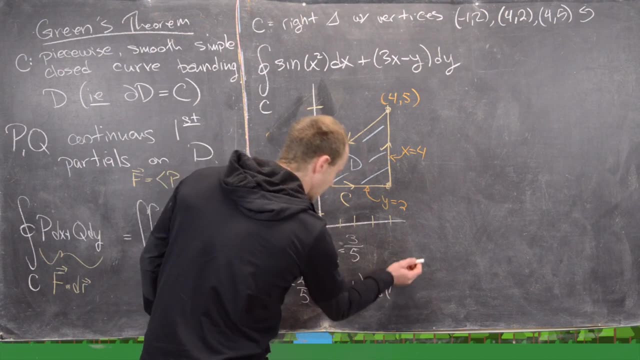 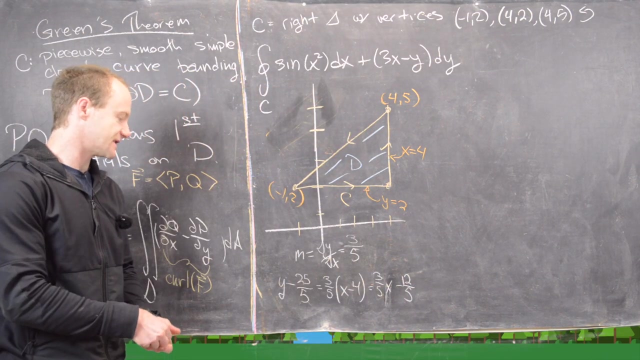 be equal to 3 fifths, and then x minus the x part of the point, which is 4.. But now we can multiply that out. That is 3 fifths times x minus 12 over 5.. Okay, good, But now putting this all together, 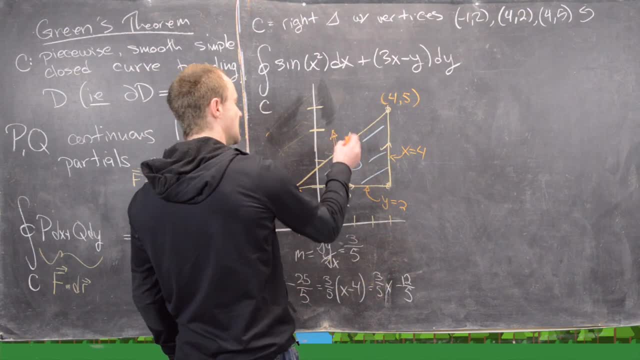 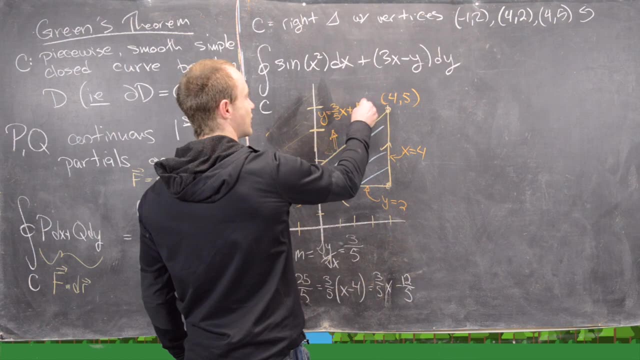 we'll get the equation of this line right here. is: given by: y equals 3 fifths x plus 13 over 5.. So that's going to be equal to 3 fifths x minus 12 over 5.. So that's going to be equal to: 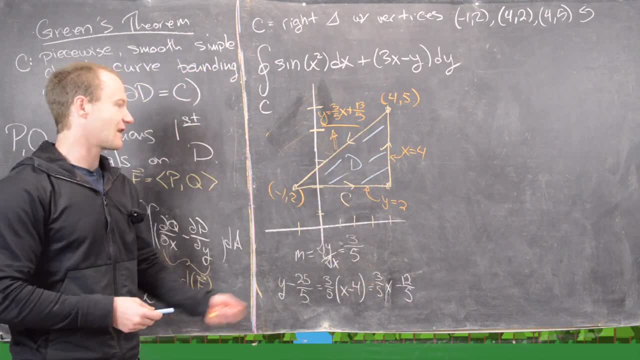 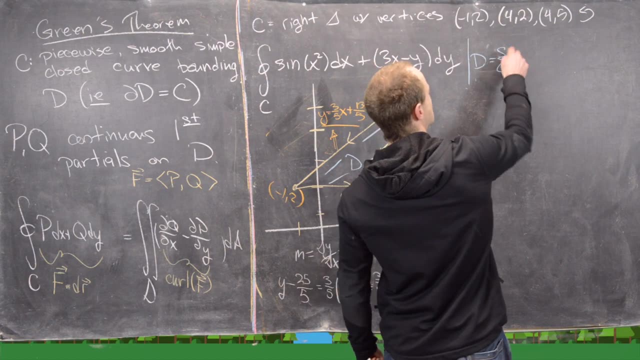 3 fifths x minus 12 over 5.. Great, But now that allows us to write this region d as a type 1 region in a pretty easy way. So notice that d is going to be equal to all points, x, y where x is running. 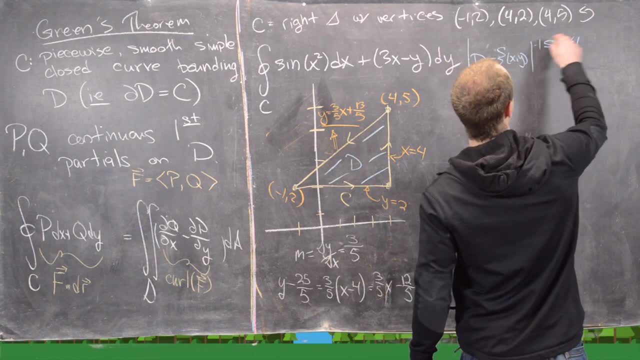 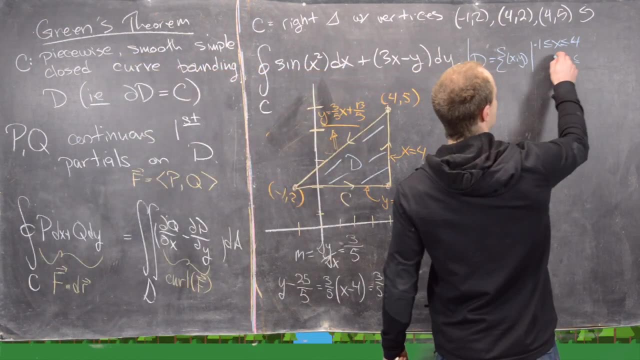 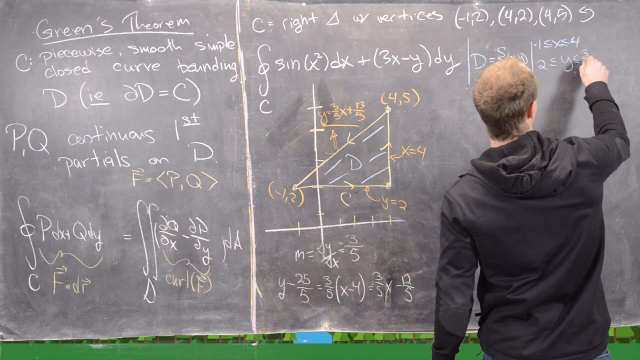 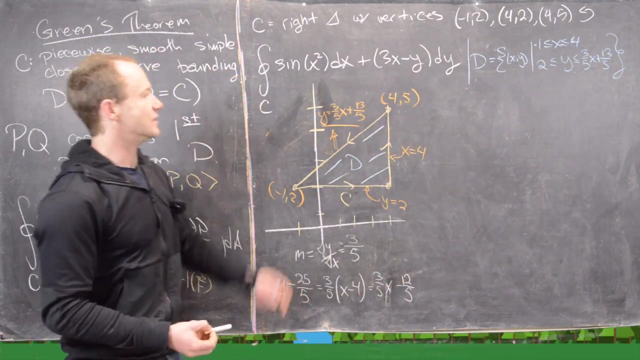 between negative 1 and 4.. So that's pretty easy to see. And then y is running between 2, which is this horizontal line down here and this slanted line up here. So that's 3 fifths x plus 13 over 5.. Good, Now what we can do is rewrite this. 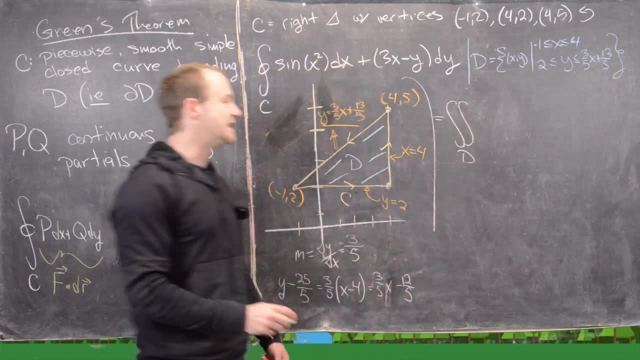 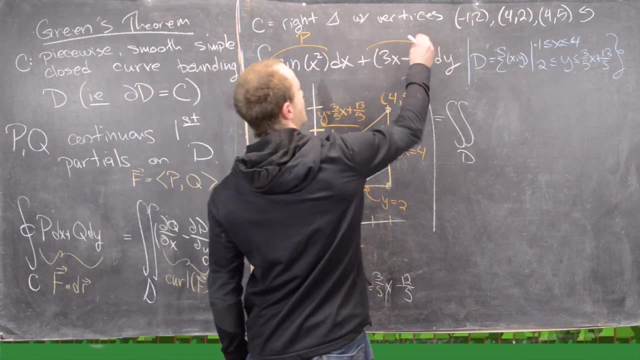 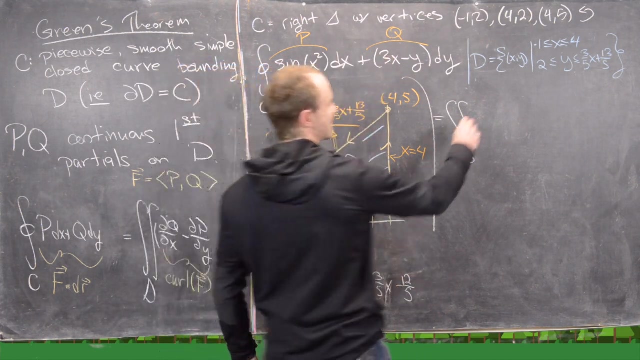 line integral as a double integral over d, using Green's theorem, where this sine of x squared is our function p and this thing, 3x minus y, is our function q. So we need partial q, partial x. but that's pretty easy, That's just: 3x minus y is our function q. So we need partial q, partial x. but 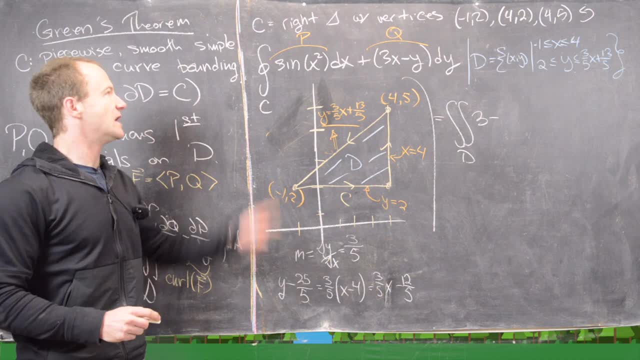 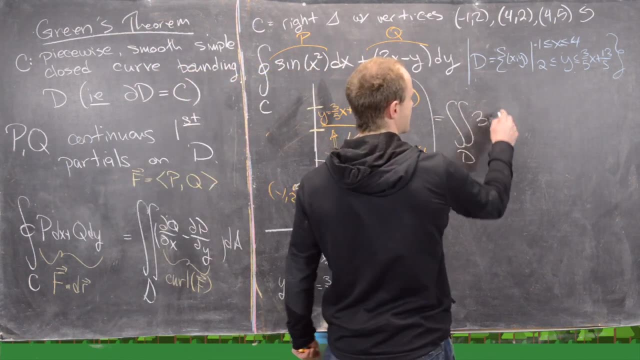 that's 3 minus partial p, partial y. But notice: partial p, partial y is 0, because there's no y's in there. Good, So I'm just going to go ahead and erase that, and we have this d a right here Now. 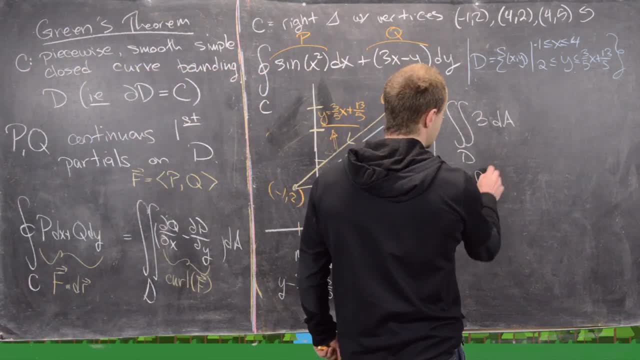 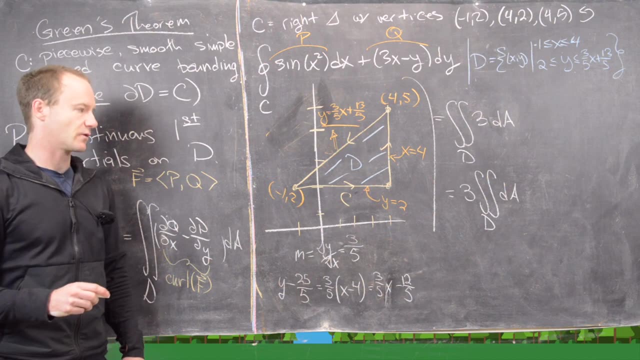 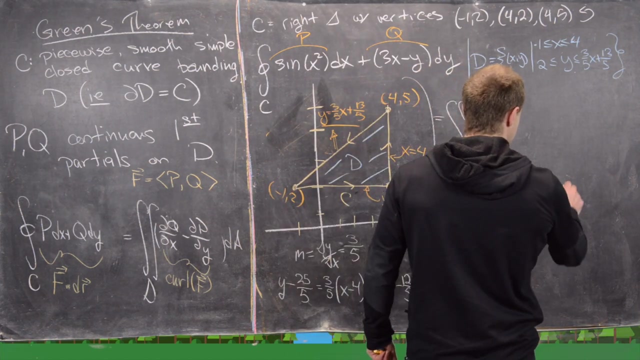 the next thing that we can see is that this is 3 times the double integral over d, d, a. And now we can actually calculate this a couple of different ways. The way I want to do it first is notice that is exactly equal to 3 times the area of the region D, because the double integral of just 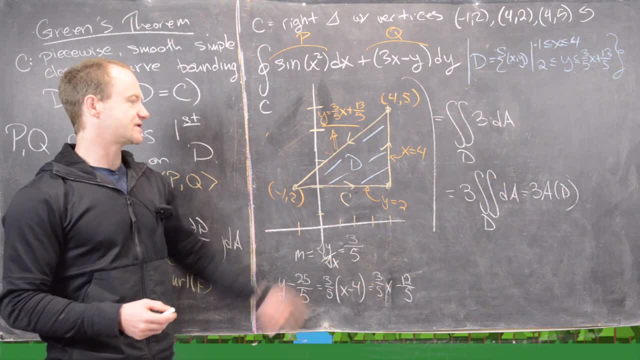 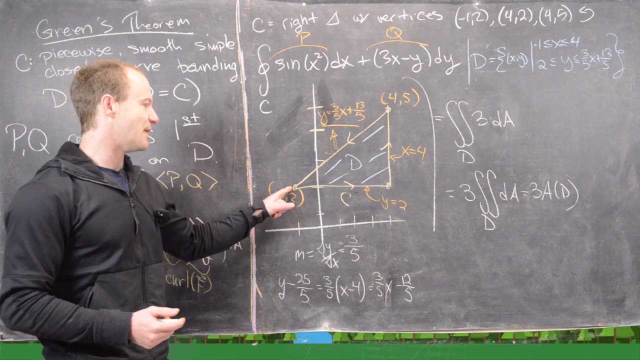 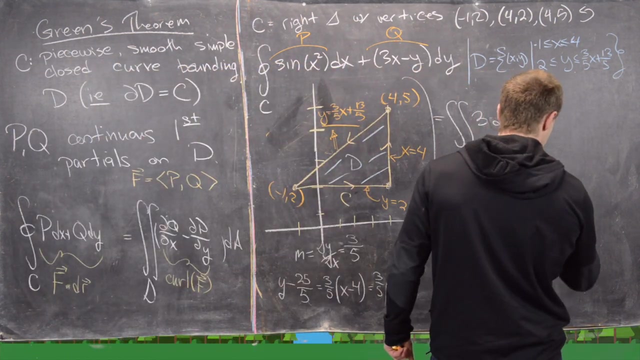 DA over. D is just the area of the region, But this is a right triangle and triangles have a well-known area formula. Notice: this has base of 5, and it has height of 3.. So this is 3 times 1 half base height. so 1 half base, which is 5, times height, which. 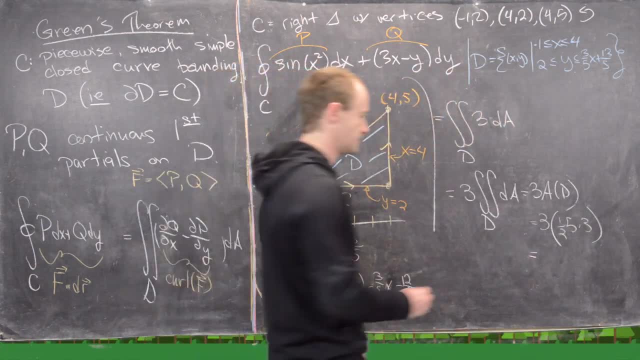 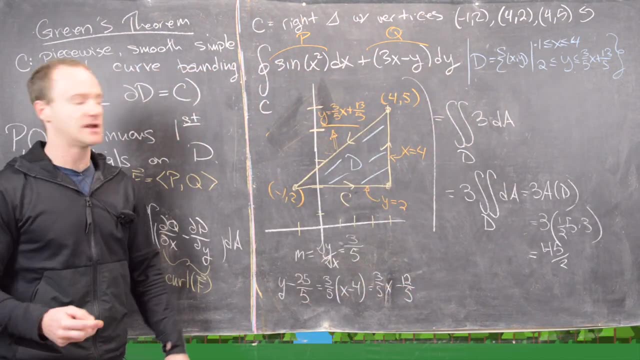 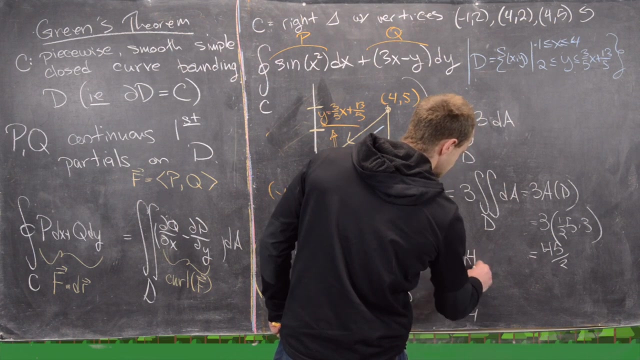 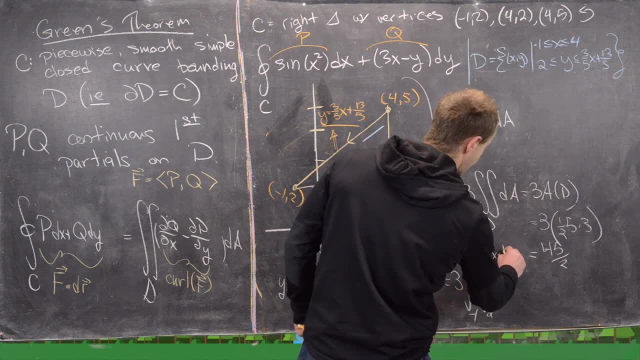 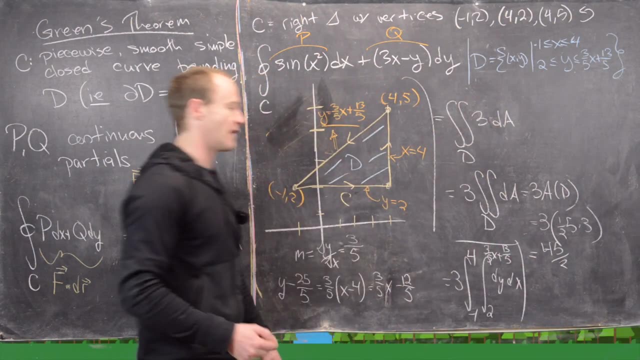 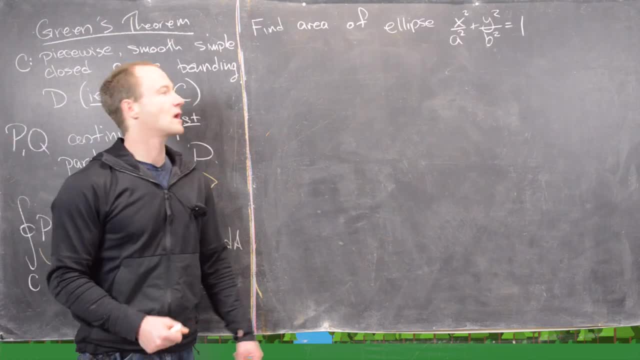 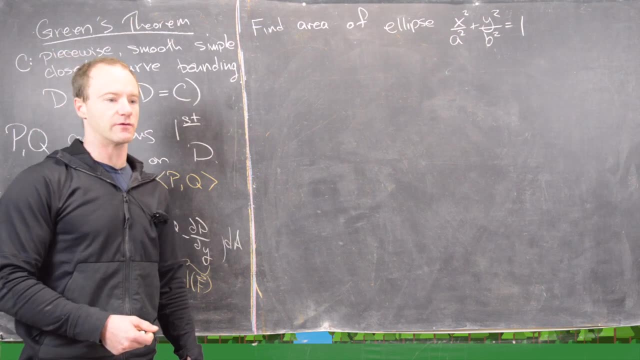 good, I'm going to clean up the board and we're going to do another example. Okay, for our next example, we're going to find the area of an ellipse. So x squared over a squared, plus y squared over b squared, equals 1.. And calculating this as a double integral is actually: 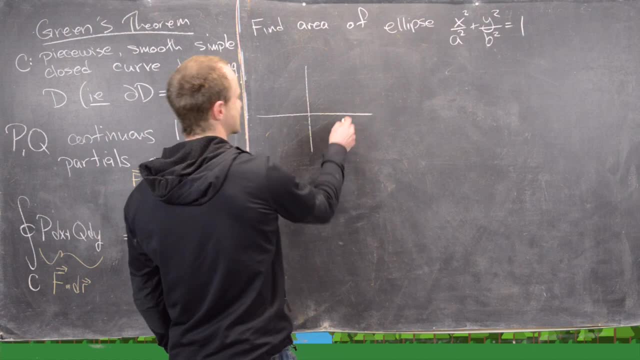 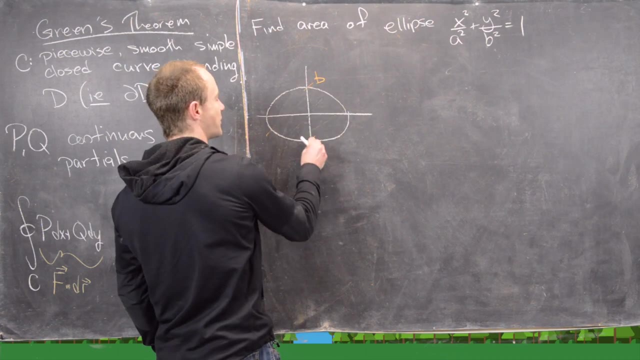 quite hard. So we're going to do another example. So we're going to do another example And, you know, let's maybe sketch out why that's the case. So notice, an ellipse is going to have the following form: It's going to go through this point up here b, this point. 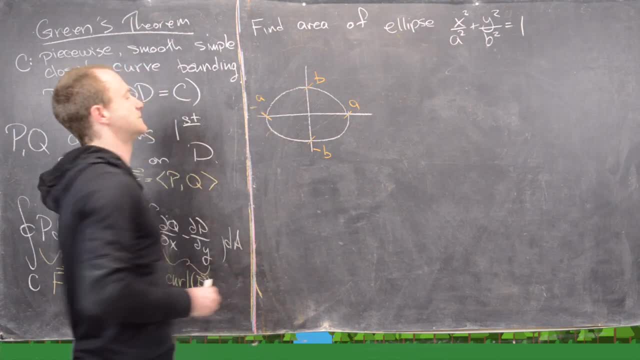 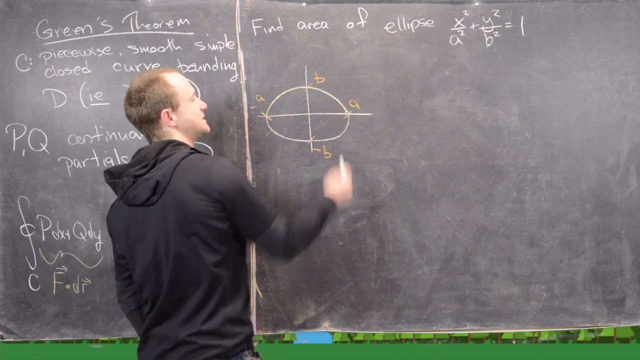 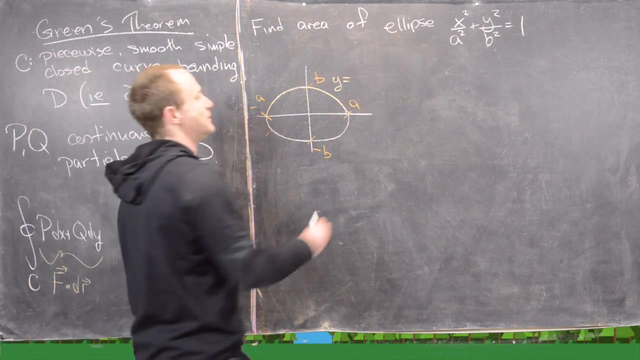 down here negative b, here a and negative a, And notice we can maybe write this top half of the ellipse as y equals. so we can solve that for y And let's see what we'll get. We'll get b squared minus y squared over b squared, plus b squared over b squared. 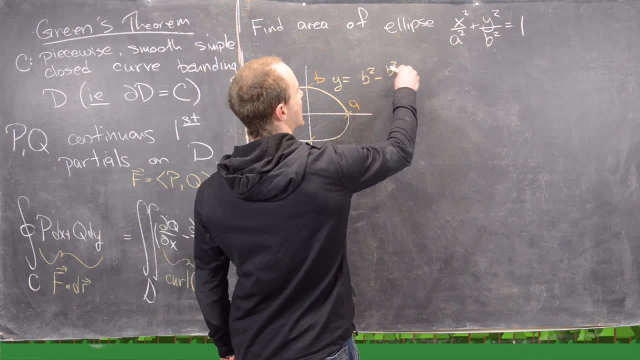 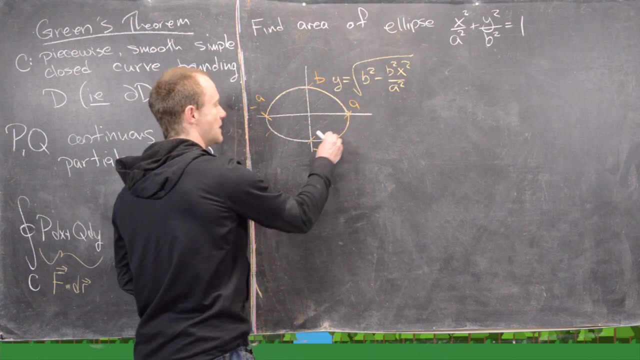 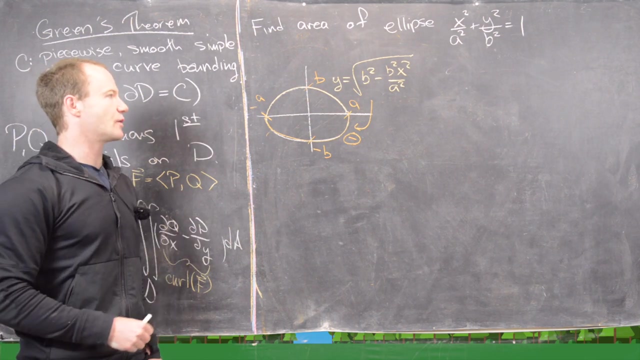 minus b squared x squared over a, squared the square root of that thing, and then down here in the bottom half, we'll get the same thing, but with a minus sign, and so I urge you to write down what the double integral for this area would be, but I will tell you that it will be pretty. 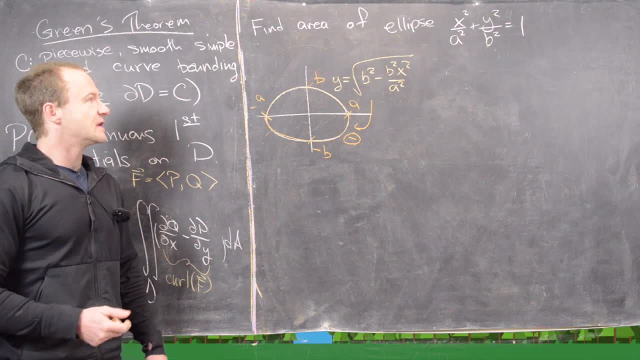 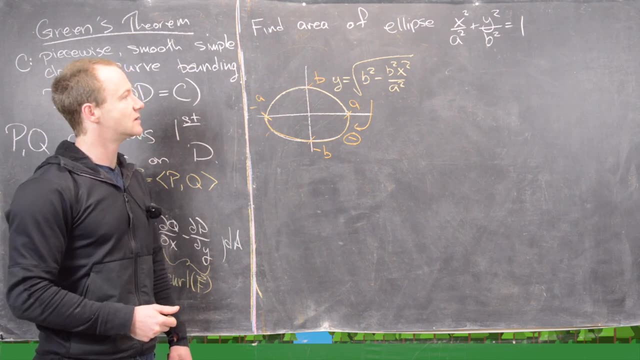 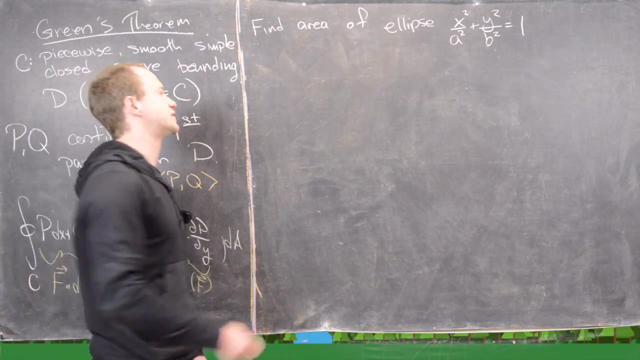 difficult to calculate and maybe not worth it. so we're actually going to take a little bit different of an approach in order to do that. so I'll erase this picture and then we'll get started with our other approach. Okay, so our other approach is to use green's theorem. so 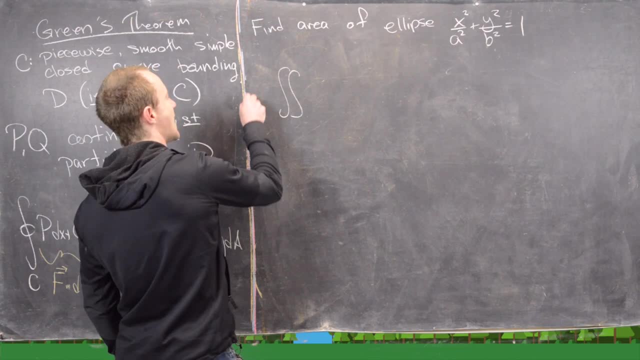 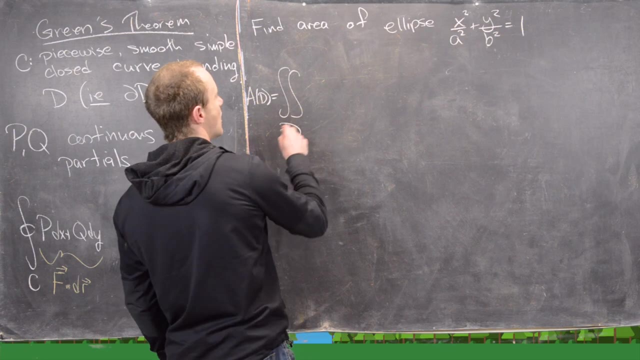 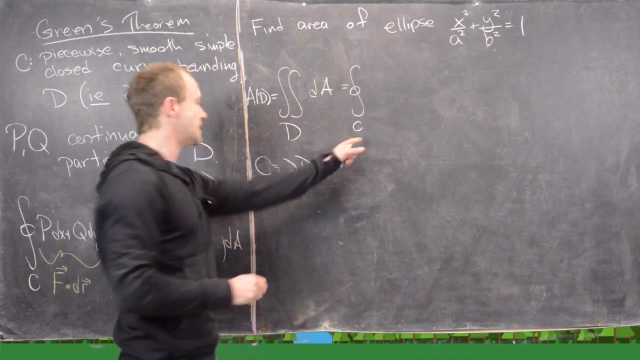 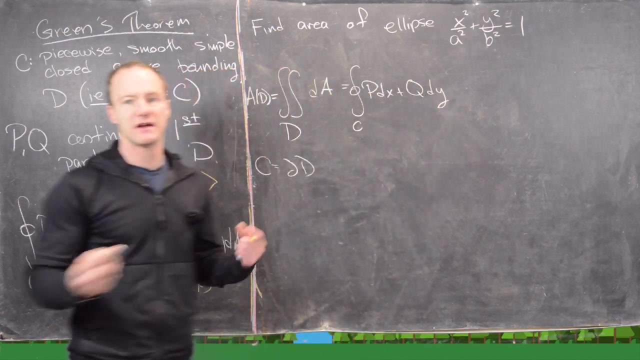 what we need to do is to notice that we have the area of d, where we'll call the ellipse: d is going to be equal to the double integral over just da, but now we can rewrite this as a line integral over c, where c is the boundary of d, of pdx plus qdy. but there have to be very, very special. 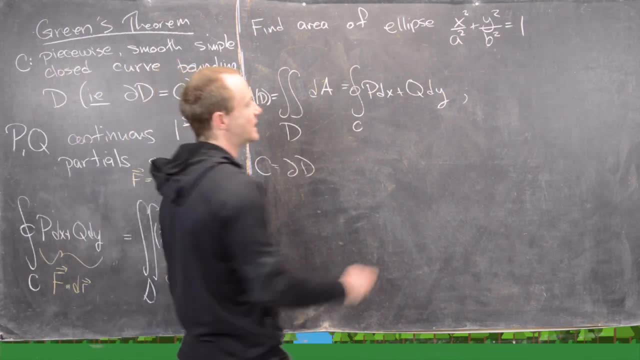 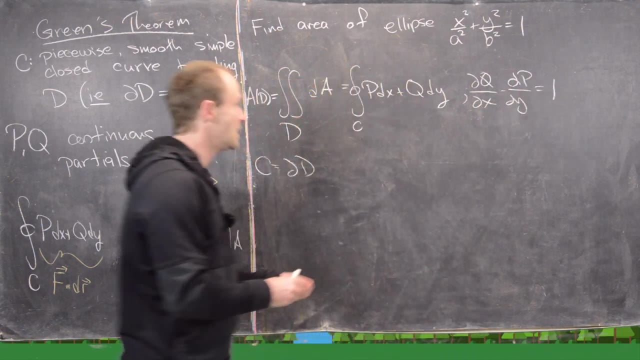 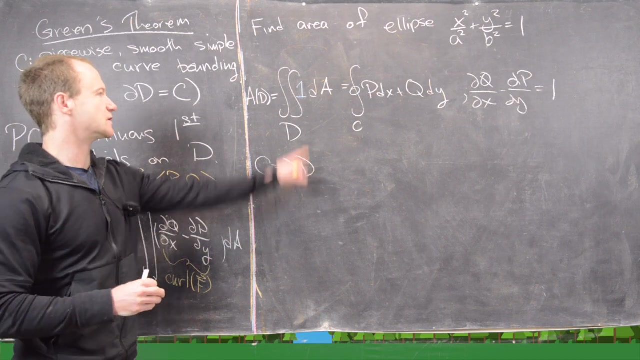 choices of p and q. In fact, what we need is partial q, partial x minus partial p, partial y equals one, because we can apply Green's theorem to this right-hand side, and if that difference of those partials equals one, then the left-hand side is exactly what we want And then also notice. 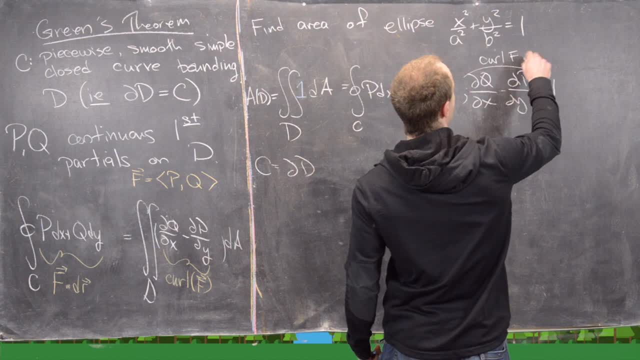 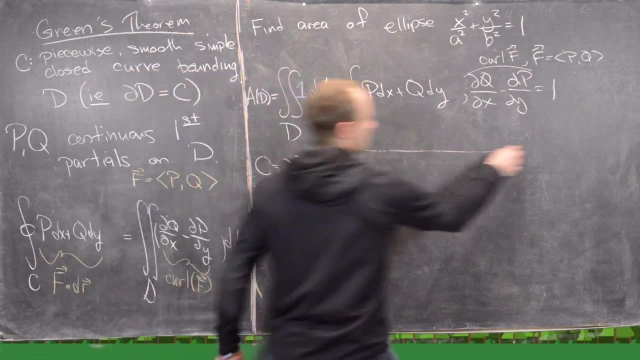 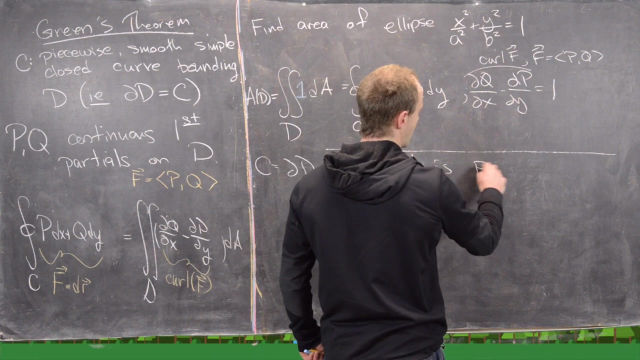 that this is equal to the curl of f, where f is the vector field made by p and q. So maybe this builds. a really important question is: what is a good choice for our vector field f, which is p, q? So 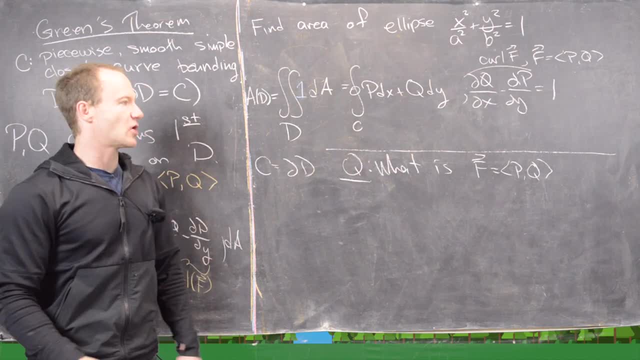 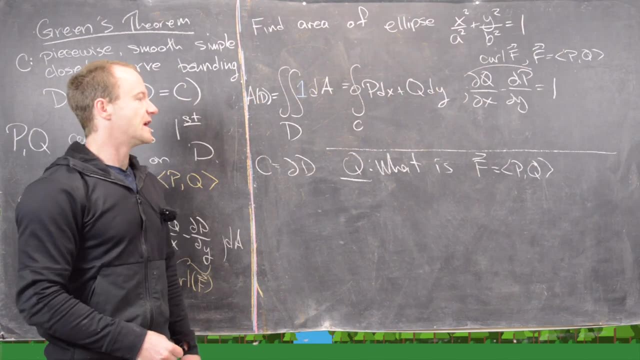 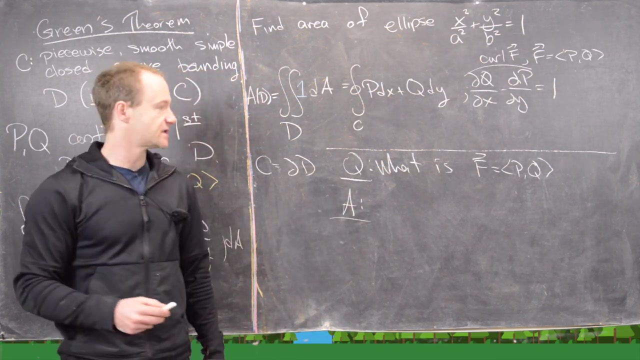 just to reiterate, what we want is partial q, partial x minus partial p, partial y to be one, or in other words, the curl of f needs to be one. Okay, and so, to answer this question? well, there are actually a lot of answers, but maybe a couple of the classic ones are the following: 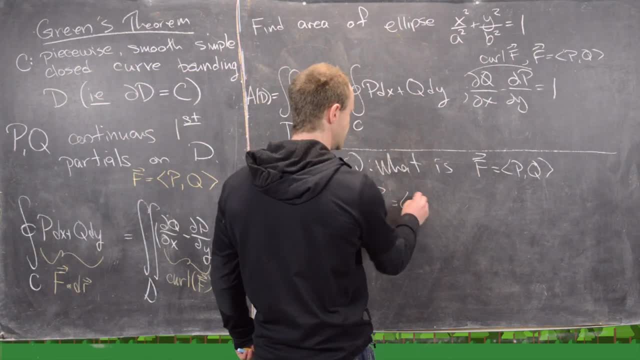 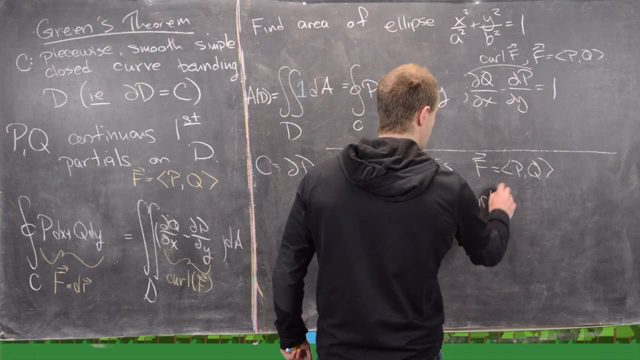 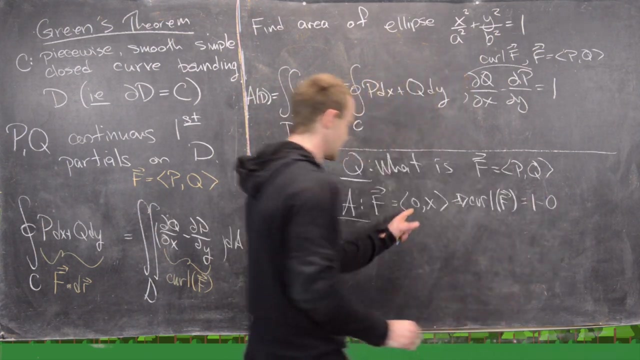 So we can take f to be equal to zero comma x, because, notice, what we get here is the curl of f. So we can take: f is equal to the partial of x with respect to x, which is one, minus the partial of zero with respect to zero, which is zero, so we get one. So we get what we want. Or we can take f to be equal to negative y comma zero, but that's going to give you the same curl, because, notice, here we've got a built-in minus sign, so partial p, partial y, in this case, will be negative one, but we're subtracting it, so we have zero minus negative one, So we get one. 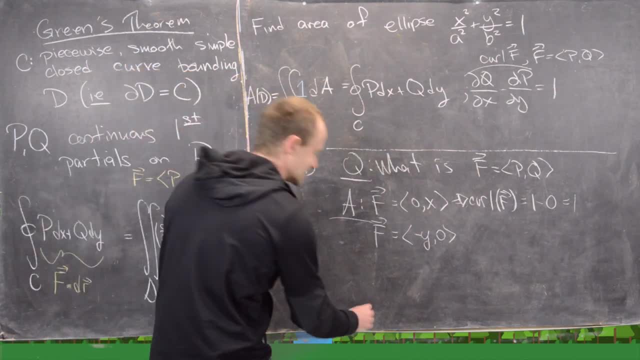 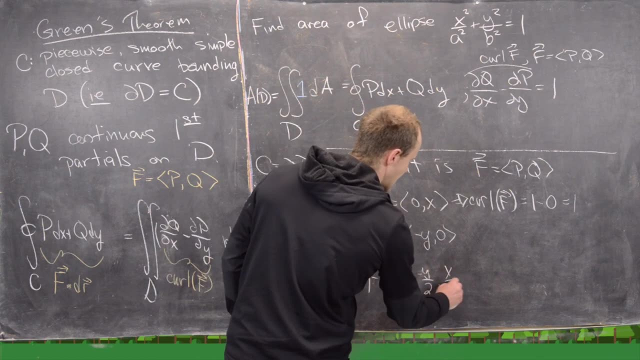 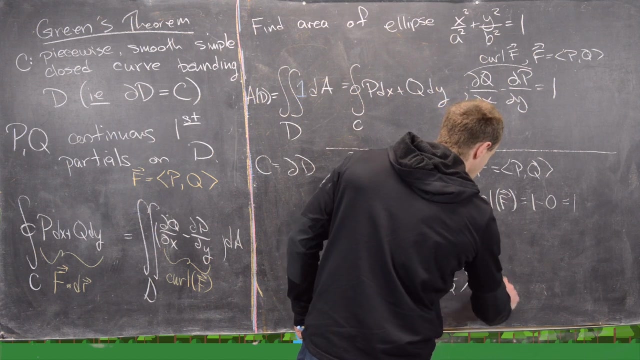 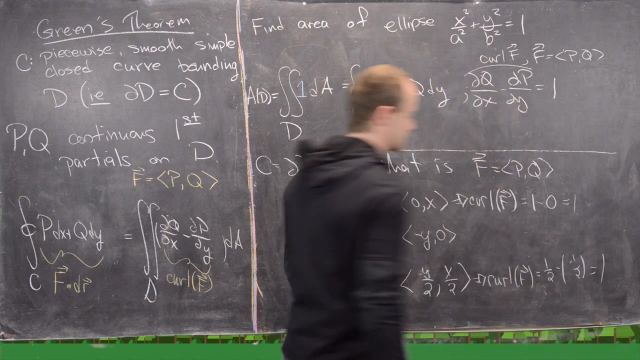 So that'll give you one. Or we could look at like a symmetrized version of this, and what I mean by that is we could take minus y over two and then x over two. But now, if we calculate the curl, in this case we will get one half minus negative one half, which is equal to one. 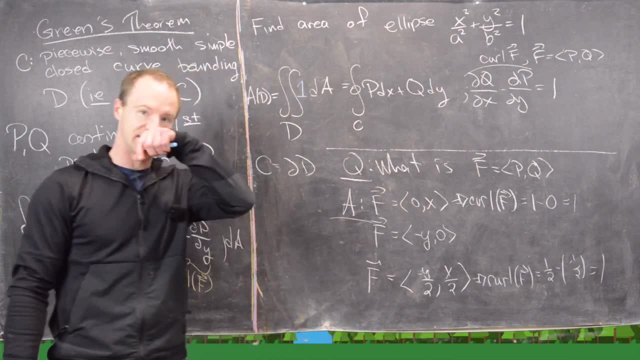 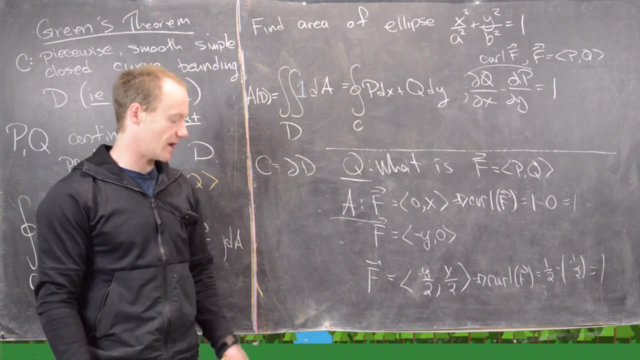 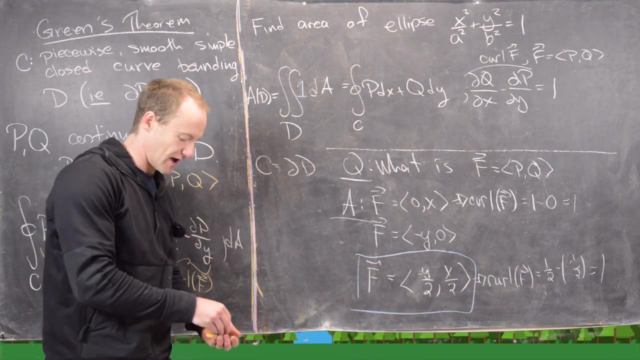 And that's easy to check. The partial of this guy with respect to x is half of this guy with respect to x is negative half. you put those in there. one minus negative half is one and in fact this is the right version and I'll let you guys maybe like play around with these. 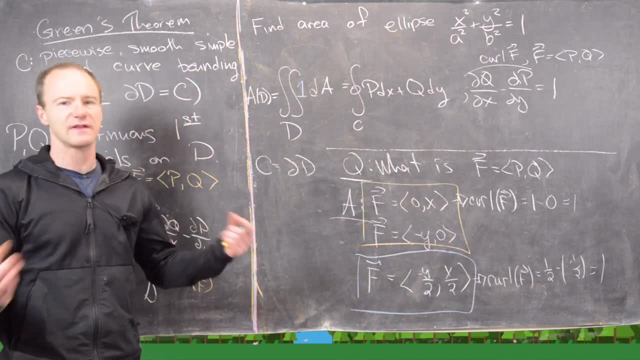 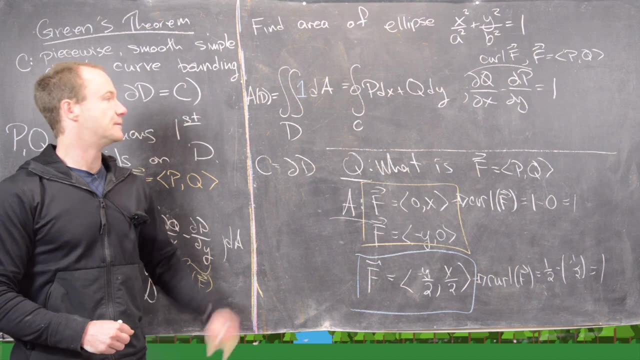 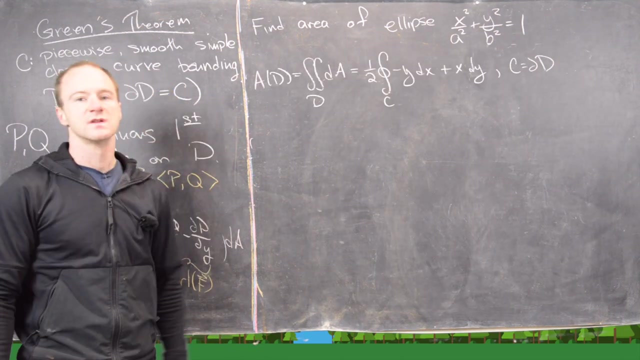 versions, and if you do that, you see, you'll get something that is definitely solvable, but it's easier to do with the one that I've, uh, squared in blue. okay, so, um, I'm gonna clean up the board and then we're going to proceed with this. okay, on the previous board, we argued via green's theorem. 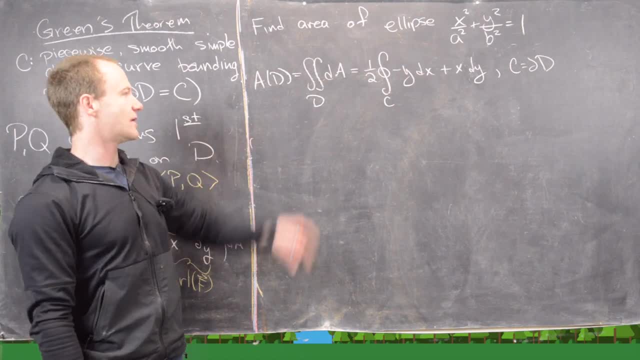 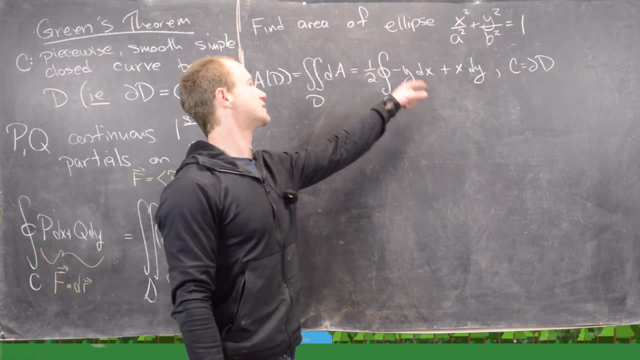 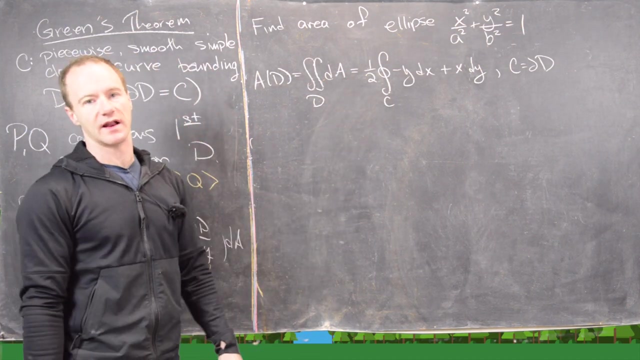 that we can take the area of a region, d, which is the double integral of da over d, and write that as one half the line integral over c of minus y, dx, plus x, dy, where c is the boundary of d. and I've taken this one half out of the line integral, kind of just to make it a little bit. 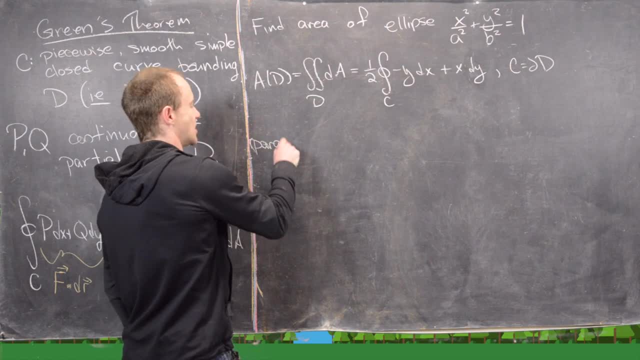 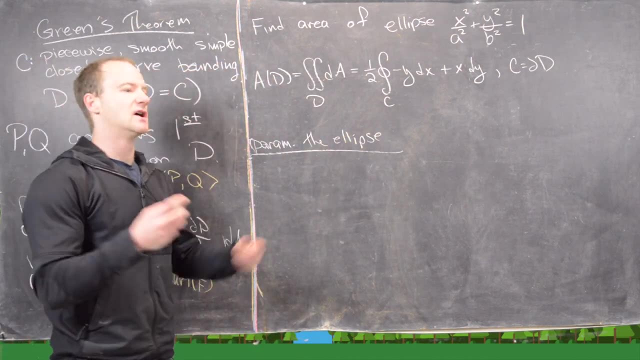 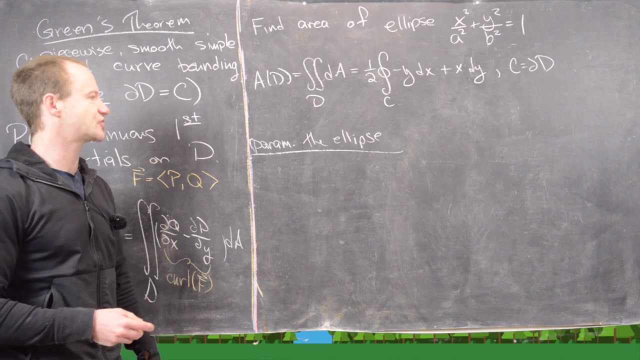 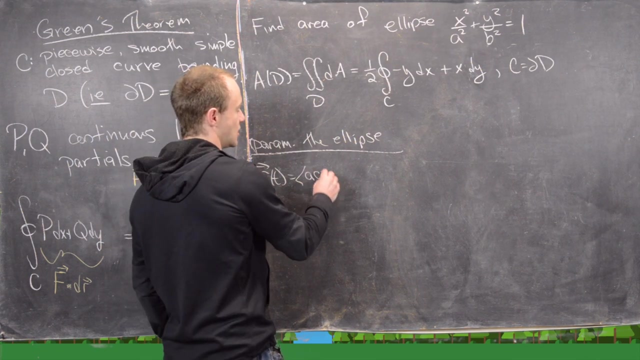 simpler. now. the next thing we want to do is uh parametrize the ellipse, and I won't labor this too much because we've done this uh much previously when we were looking at um calculus of like vector functions and parametric equations and stuff like that. but what works is: we'll take r of t to be equal to a cos t, b sine t, and here t. 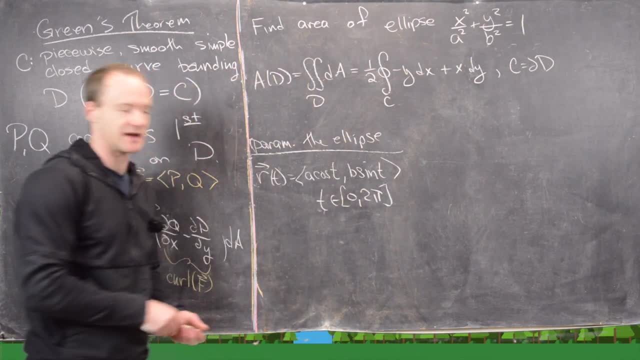 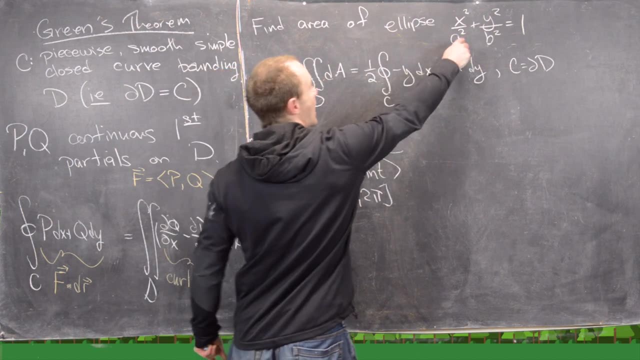 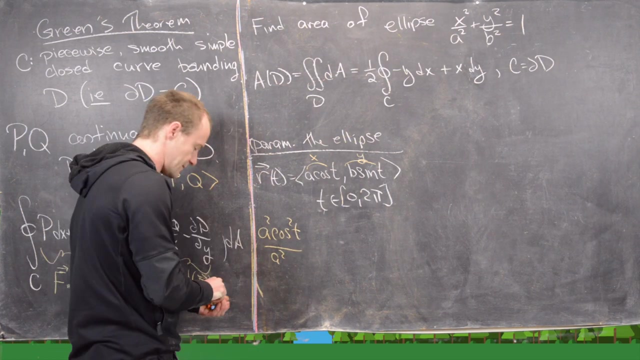 needs to run from zero to two pi in order to draw the entire ellipse. so let's just check that. real quick notice: if we plug this in for x and this in for y into our equation of our ellipse, we get a squared cos squared over, a squared plus b squared sine. 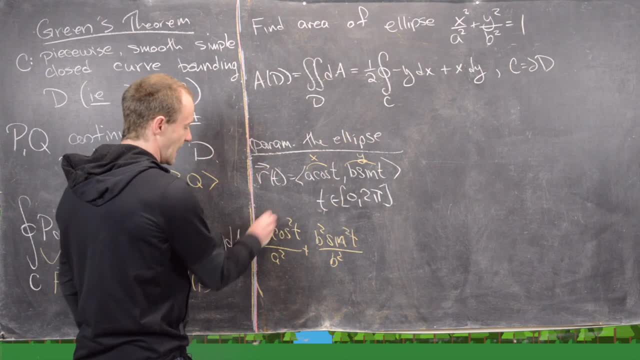 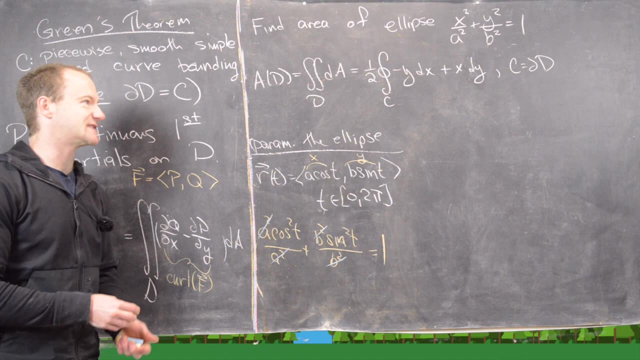 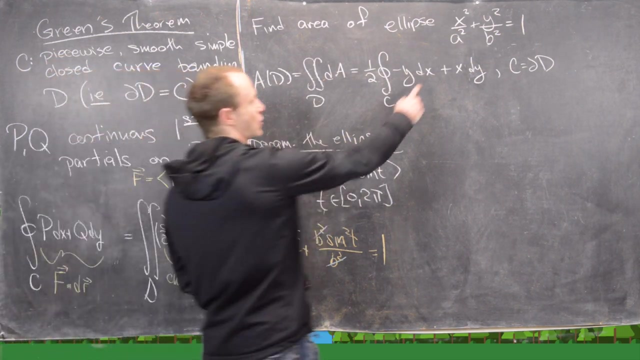 squared over b squared, but the a squareds and the b squareds cancel, which means that this turns into one, and so these do satisfy the equation of the ellipse. now, the next thing that I want to calc want to notice, is that these portions of the line integral 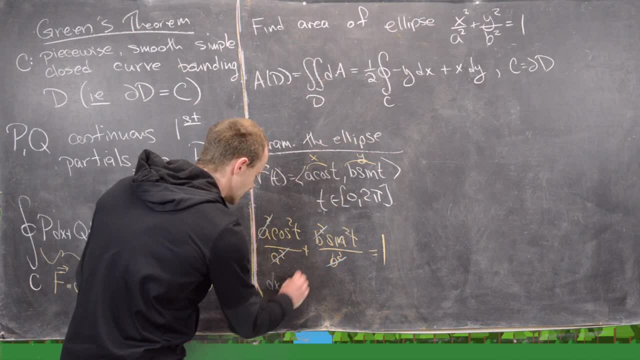 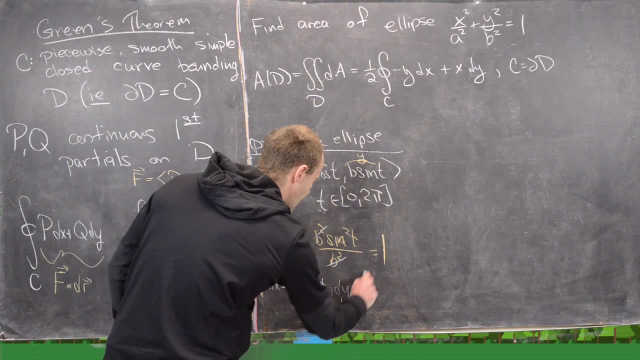 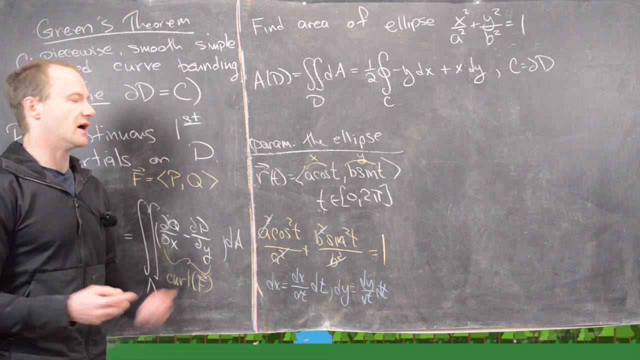 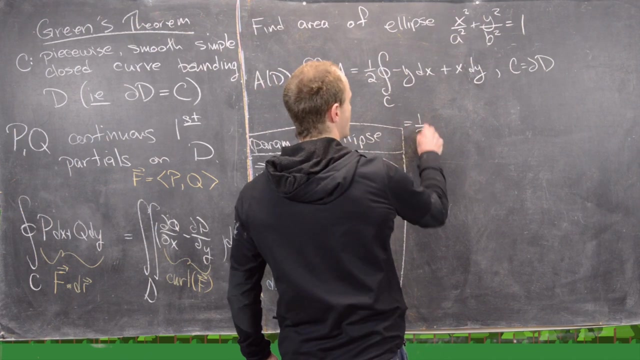 dx, dy, uh, can be written using the following rule: so dx is dx, dt, dt, and likewise dy is dy, dt, dt. so just recall that from when we were calculating um line integrals for their own sake. okay, great, now we're ready to go ahead and calculate this. notice. this is going to be one. 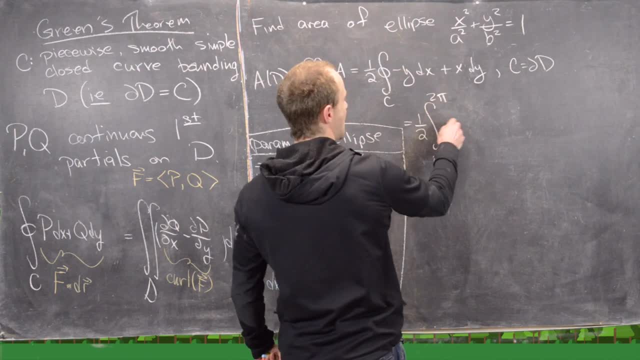 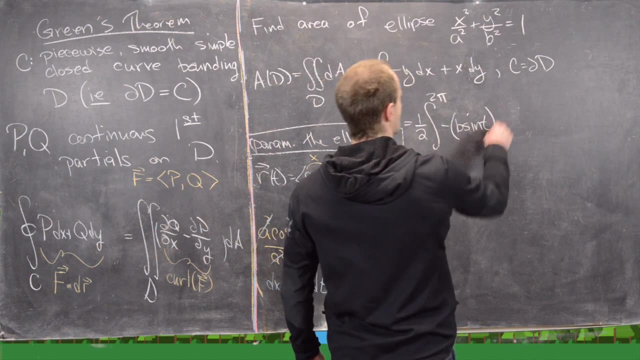 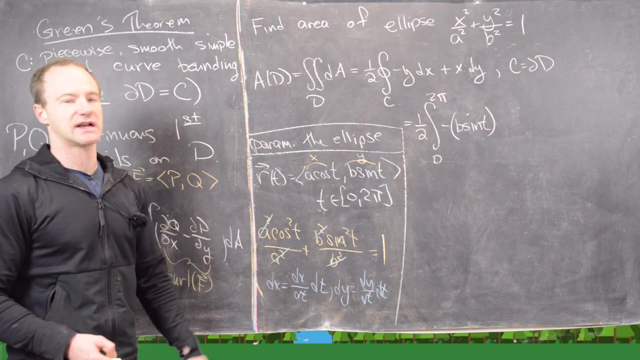 half the integral, from zero to two pi. and then we have minus our y component, so that's going to be b sine t. and then we have our dx component. so notice, our dx component will be the derivative of a cosine t, so that's going to be minus a. 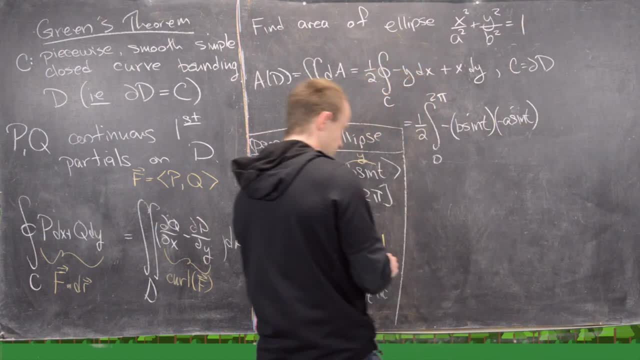 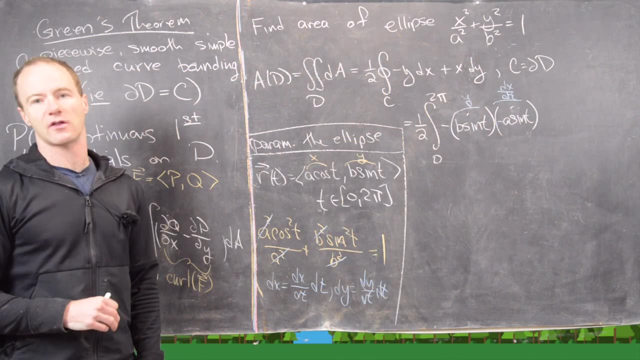 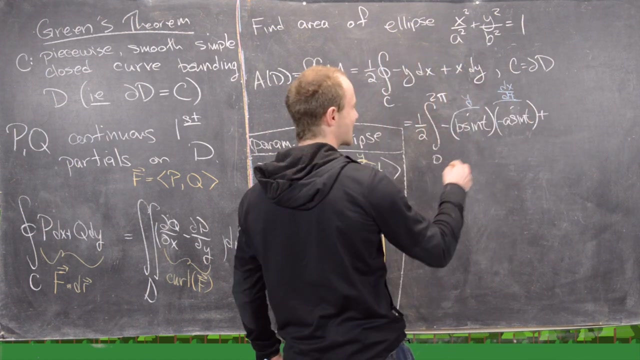 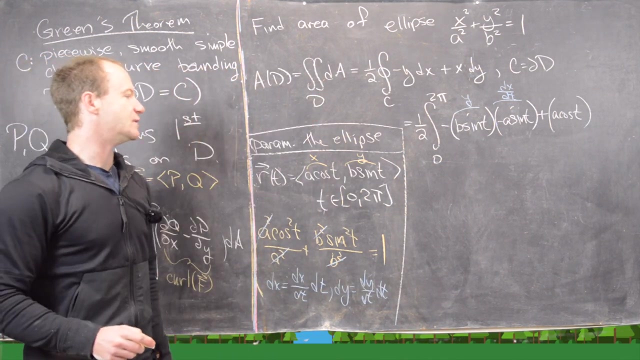 sine t. so just to point this out, this is our y and this is dx, dt. I'm going to factor uh dt out of the whole right hand side, so let's hold off on that. and now we're going to add to this x, but notice, x is a cosine t from this term right here. and then dy, but that is going to involve dy, dt.